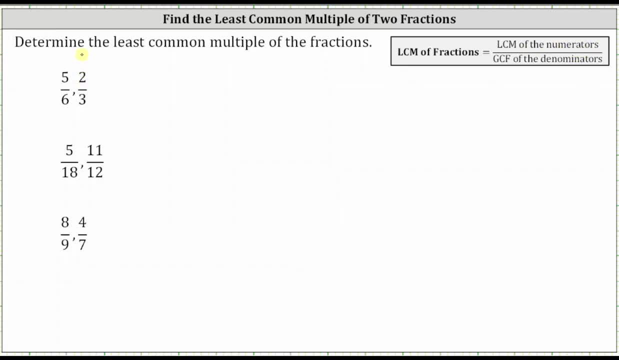 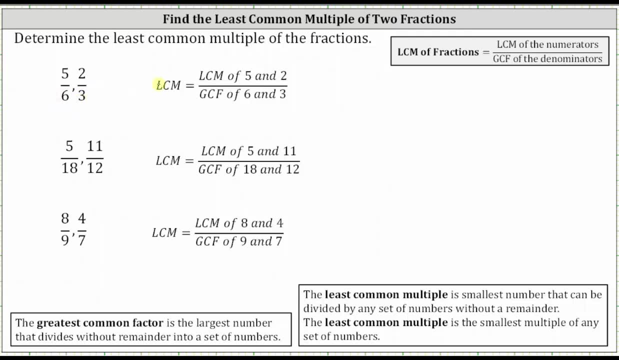 Let's look at some examples. We want to find the least common multiple of each pair of fractions. So to set this up, to find the least common multiple of five, six and 2, 3rds, we need to find the fraction. 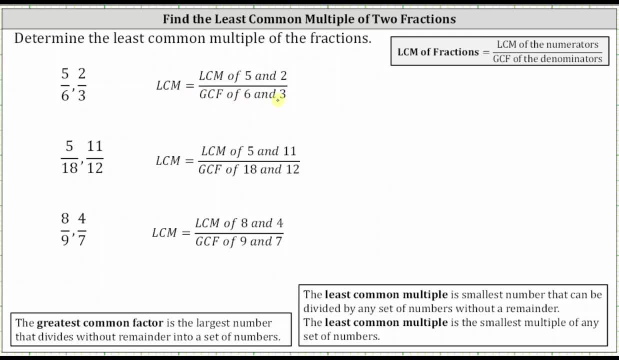 where the denominator is the greatest common factor of six and three and the numerator is the least common multiple of five and two. Now I do have other videos that show how to determine the greatest common factor and the least common multiple, but for review, the greatest common factor: 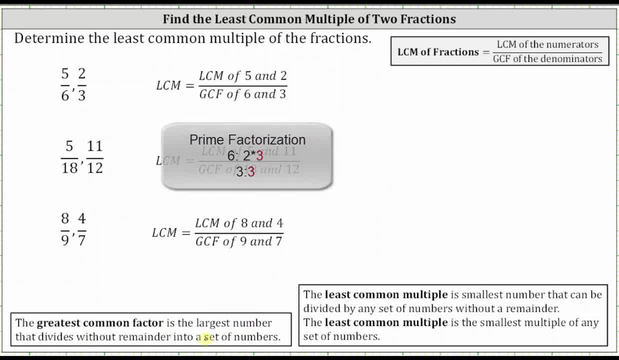 is the largest number that divides, without remainder, into a set of numbers. So the greatest common factor of six and three is the largest number that divides both six and three without remainder, which is three. Six divided by three is two. three divided by three is one. 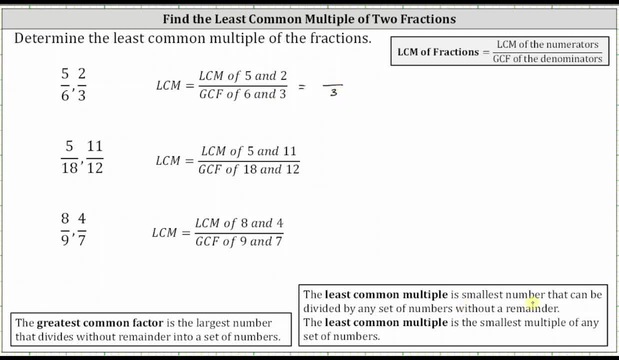 And the least common multiple can be thought of in two ways. It's the smallest number that can be divided by any set of numbers without remainder. It's also the smallest multiple of any set of numbers, So the least common multiple of five and two. 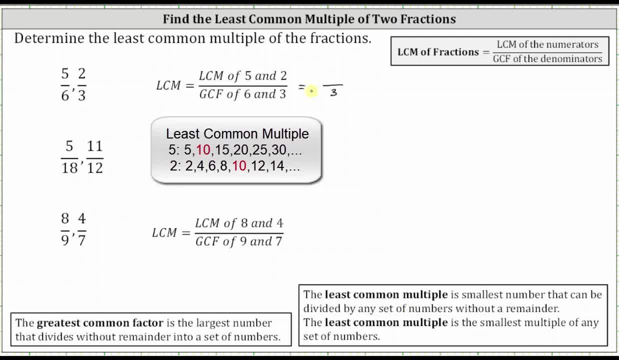 is the smallest number that can be divided by both five and two, which would be five times two or 10.. 10 is also the smallest multiple of both five and two. 10 thirds is the least common multiple of five, six and two thirds, which means 10 thirds is the smallest. 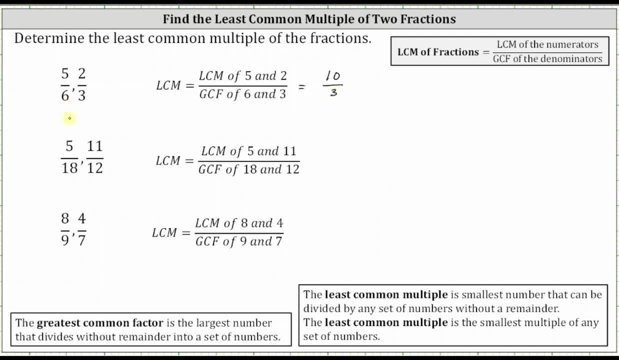 fraction that can be divided evenly by both five, six and two thirds. It's also the least or smallest multiple of both fractions. Next, we want to find the least common multiple of five, eighteenths and 11 twelfths, which is equal to the fraction where the denominator 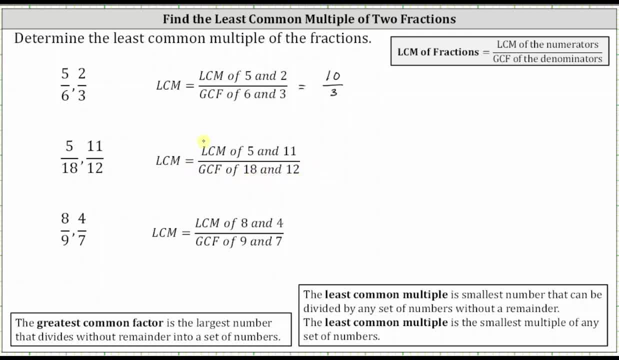 is the greatest common factor of 18 and 12, and the numerator is the least common multiple of five and 11.. So the greatest common factor of 18 and 12 is the largest number that divides both 18 and 12, without remainder, which would be six. 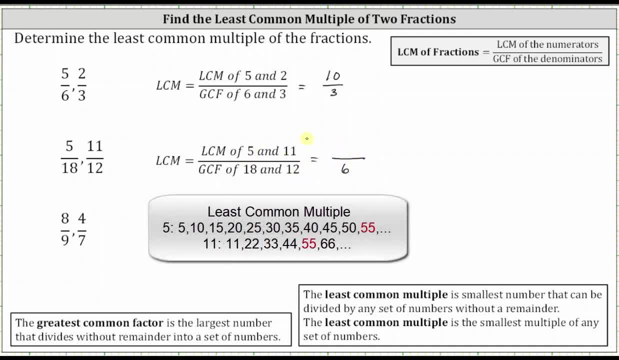 And the numerator is the least common multiple of five and 11,, which is the smallest number that can be divided by both five and 11.. And since five and 11 only share a common factor of one, five times 11, or 55, is the least common multiple. 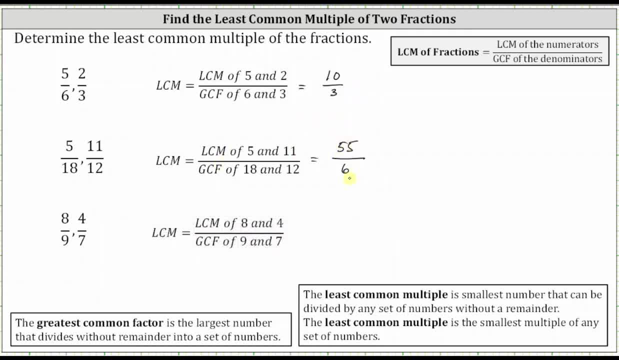 of five and 11,, which means 55, six is the least common multiple of five and 11.. So it's the least common multiple of five eighteenths and 11 twelfths. 55, six is the smallest fraction or smallest number. 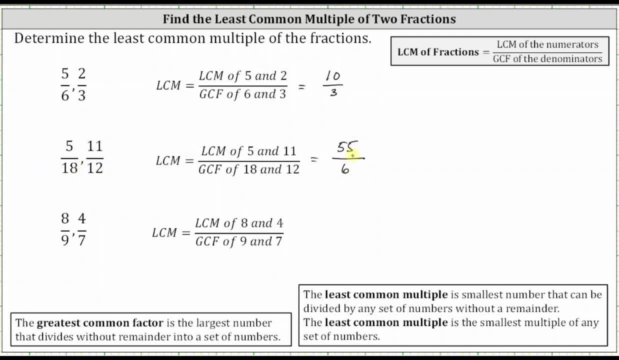 that is divisible by both fractions and it's also the smallest multiple of both fractions. For the last example, we want to find the least common multiple of eight, ninths and four sevenths, which is equal to the fraction where the denominator is the greatest common factor of nine and seven. 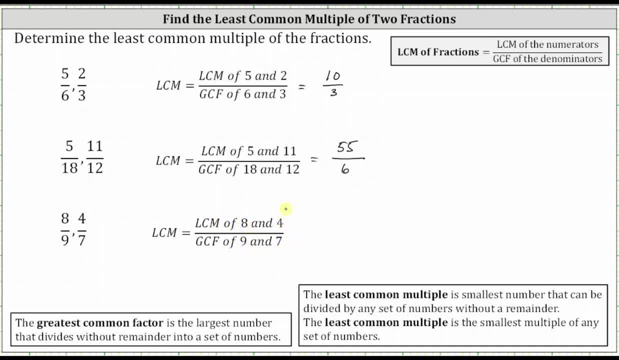 and the numerator is the least common multiple of eight and four. So the greatest common factor of nine and seven is the largest number that divides both nine and seven without remainder, While nine and seven don't share any common factors other than one, the greatest common factor. 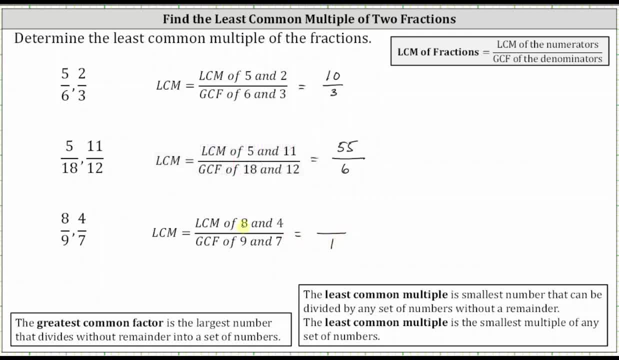 of nine and seven is one, The least common multiple of eight, and four is the smallest number that can be divided by both eight and four, which would be eight. Notice here: eight over one simplifies to just eight. Eight is the least common multiple of eight. ninths: 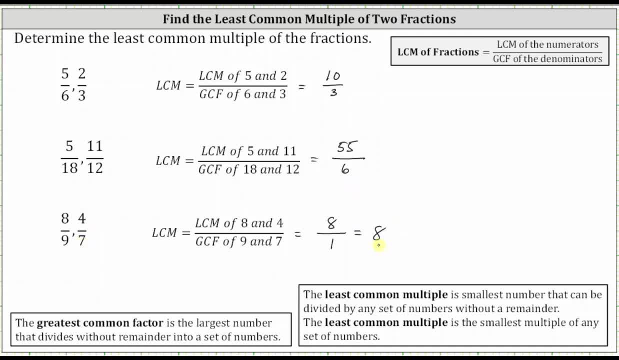 and four sevenths, which means eight, is the smallest number that can be divided by both eight ninths and four sevenths, and it's also the smallest multiple of both fractions. I hope you found this helpful. 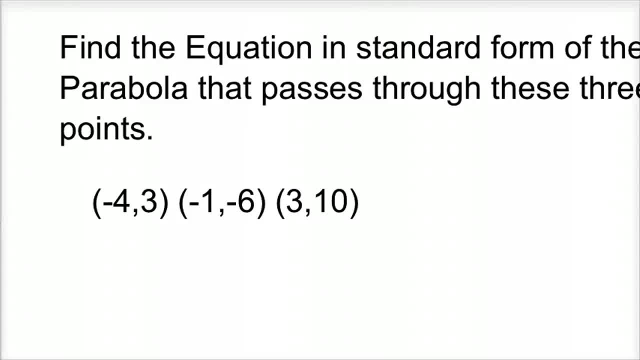 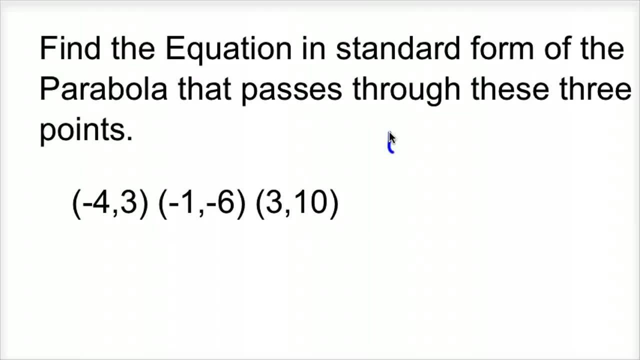 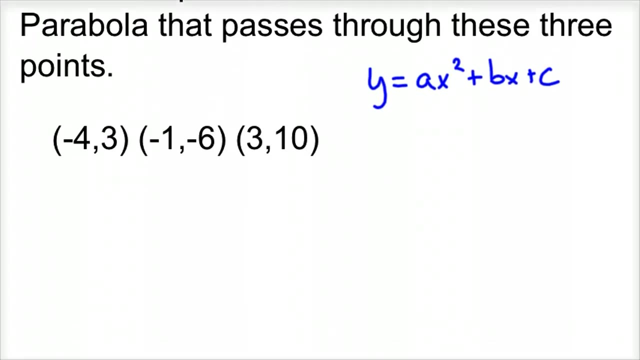 So here's how you find the equation of standard form of the parabola that passes through these three points. Well, first off, the equation of any parabola, just generally, is: y equals ax squared plus bx plus c. So what we do in this case is plug in those three points. so we're going to end up with three equations. 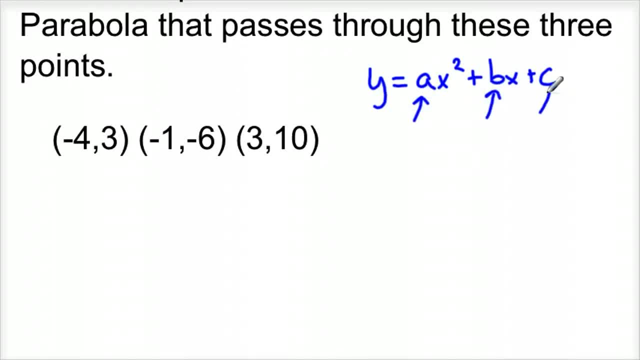 And we want to find these values. We want to find a, b and c. So I'm going to start with this first point, which is negative. 4 and 3, and plug it in, because this goes: x, y.